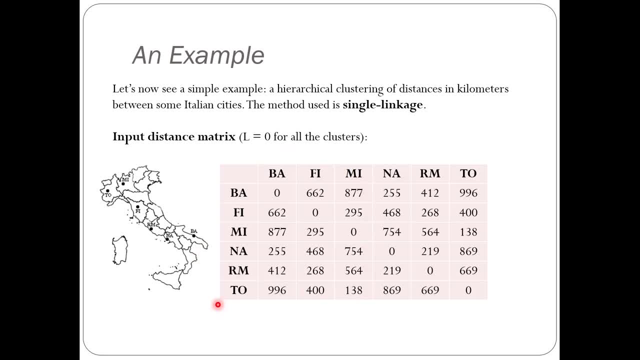 So the closest distance between cities in this case is between M, I and T? O, which is about 138.. So the first thing that we need to do is to put the observations together. The second thing that we need to do is to put these two together and form our initial cluster. 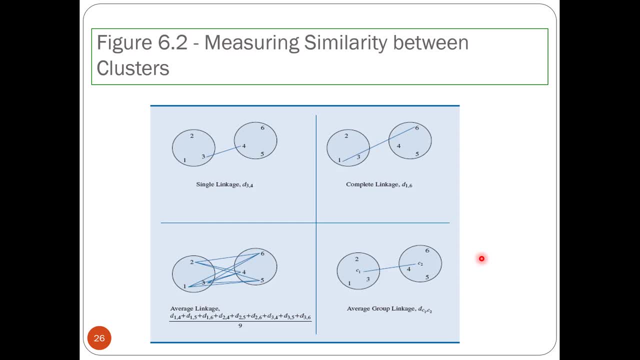 Before we get to the next step and how we update the distance matrix, I just want to give you a refresher about the way that we calculate the distances between clusters. So we have several methods to calculate distances between clusters, but the most commonly used methods are among these four. 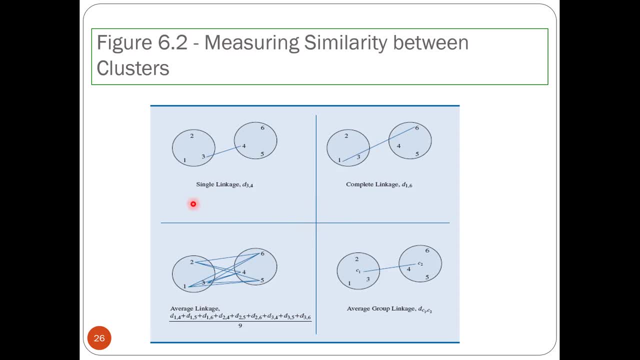 and these are the ones that are also discussed in your textbook. So the single linkage. it says: if you have two clusters, always consider the distance of these two clusters to be the shortest possible distance. So you find the two closest observations and the distance between the two closest observations. 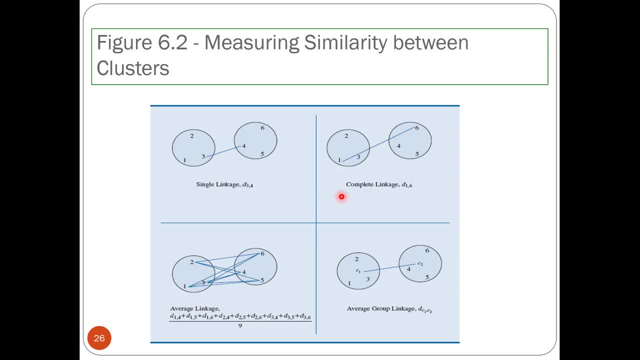 is the distance between the two clusters In the complete linkage. if you have two groups of observations, you look at the farthest distance between a pair of observations that are in two different clusters and consider that as the distance between the two clusters In average linkage. you calculate all the pairwise distances. 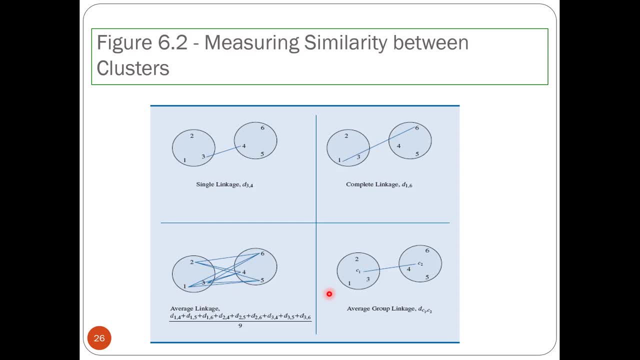 the two clusters- observations, and then calculate the average of those. and the last method, which is the average group linkage, which is to calculate the centroid of each cluster and the distances of the two centroids, becomes the measure of distance between the two clusters. This method perhaps, is one of the most commonly used methods for calculating the distance between clusters. 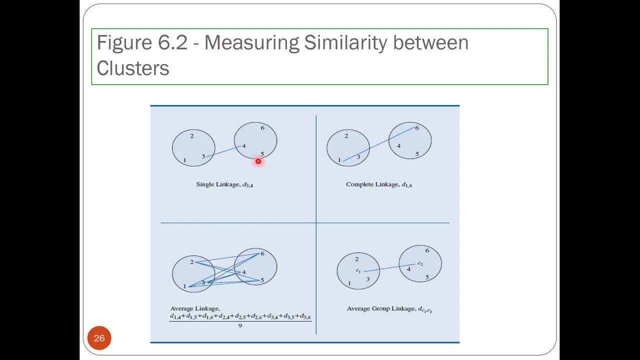 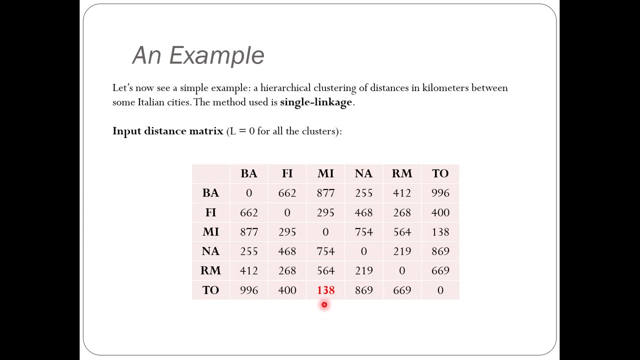 but today we're going to take a look at the single linkage. Basically, we want to look at the closest distance between the two clusters. observations as the measure of distance between the two clusters. So, if you remember, we said that TOMI and our matrix of distances have the closest distance. 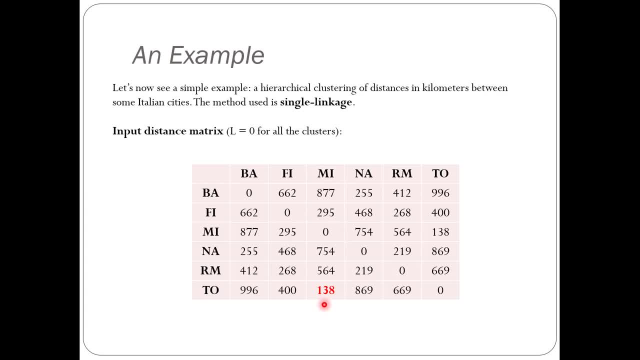 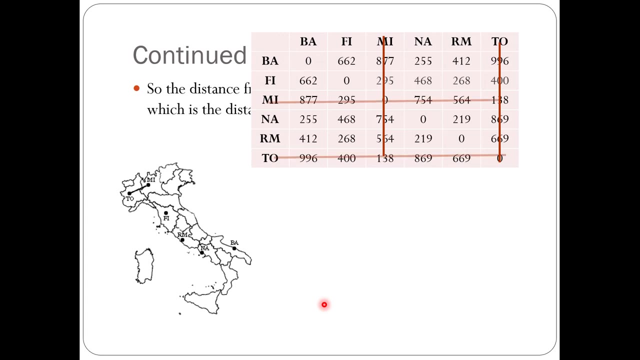 Now is the time to update our distance matrix. This time we have to combine MI and TO as a new cluster and update the distances from this cluster. This is our initial matrix. We have to remove MI and TO, Both in rows and columns, and then create a new matrix. where, in the new matrix, MI and TO are? 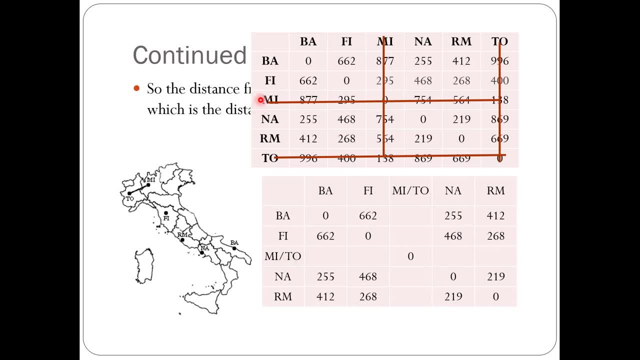 combined. So we replace the individual rows and columns and create a combined row and column for MI and TO. As you see in the left hand side, MI and TO now is combined as a new cluster. Now we have to calculate the distance of all these other observations from MI and TO. Let's get started. 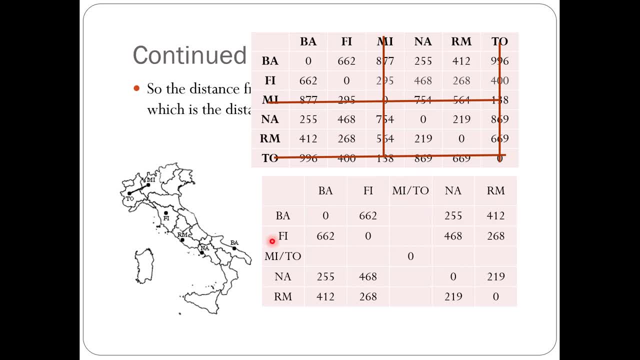 with the calculation of BA from MI and TO, We have to calculate the distance of all these other. If we go off single linkage method, we have to calculate BA's distance from these two cities and pick the closest one, because that's the principle for the simple linkage method. 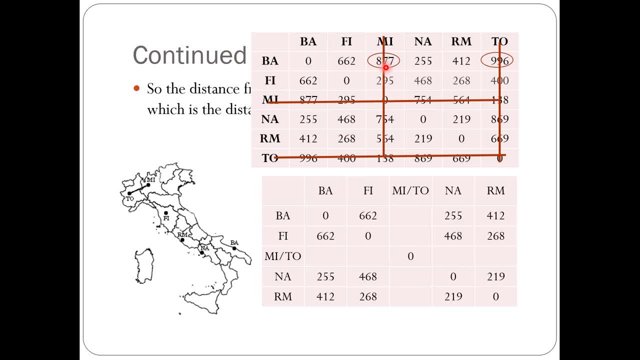 So I am looking at BA's distance to MI, which is 877,, and to TO, which is 996.. The minimum of the two sum is 877,, so the distance of BA from MI and TO is 877,. and because this is a ORE constructor. so we have to calculate the distance of BA from MI and TO. to excatantly mean the distance is MY T O, The distance of BA from MI to T O is 877, so this is the most recent distance of BA from the first lashes. and since this is also the last burst of heat, we pass the point to the HOTL and I stay next to META. Now we retention thekeiten of the bird. we have to create a hillock on the top of the cluster on tO. 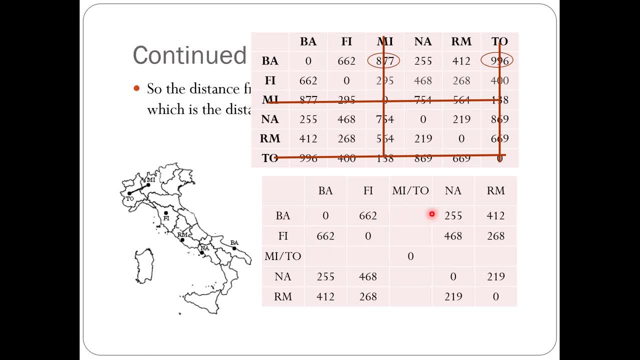 is a symmetric matrix. I can fill up both BA to MITO and MITO to BA. Now I have to find a distance from Fi to MITO. Same thing here. We look at the distance of Fi from Mi and To and we choose the minimum, And 295 is the value of the minimum of the two observations. 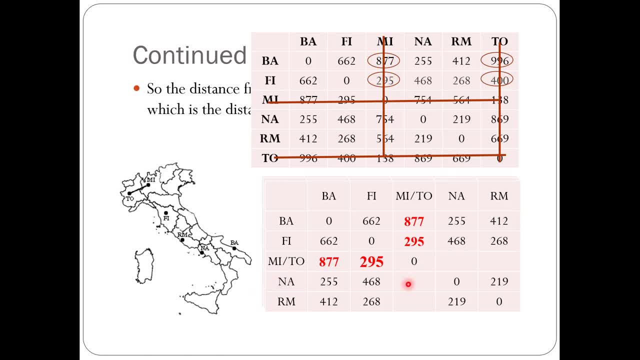 The distance from Na to MITO. Similarly, we look at the distances from Na to Mi and To and pick the minimum of the two: 754.. And for Rm from Mi and To, the minimum of the two distances is 554.. Now that we have our new, updated matrix, we can iterate the same. 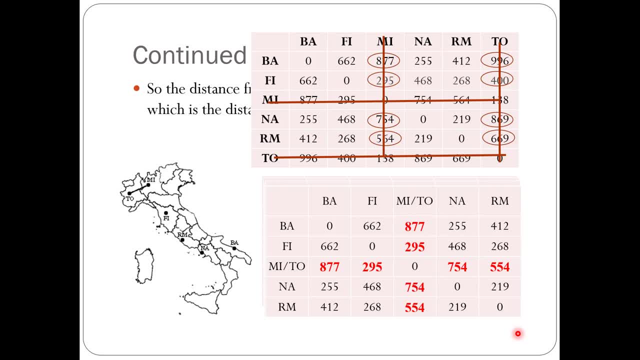 process until we get to a 2 by 2 matrix. So you have to continue this process until you have a one overarching big cluster that includes all the observations. However, as we do this process, we create a chart that we call a dendogram. Let's take a look at a dendogram. 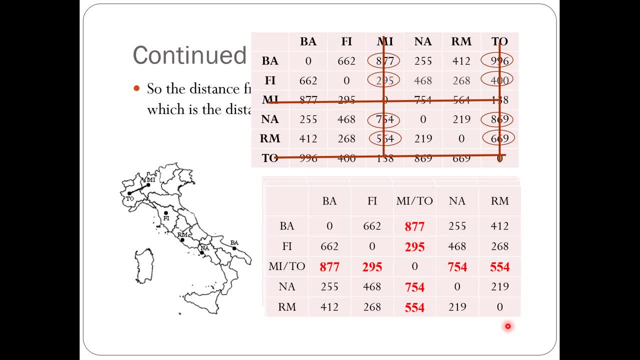 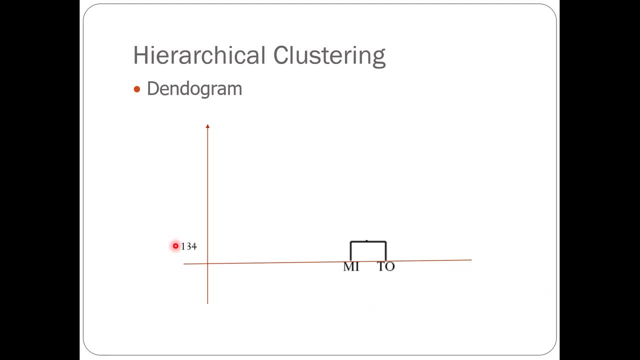 that we can create for this stage. So this is the initial dendogram that we can create. It shows Mi and To are combined and the distance between them is 134.. Now I'm going to go back to this matrix for a second, because we have to repeat the same process over and over again. 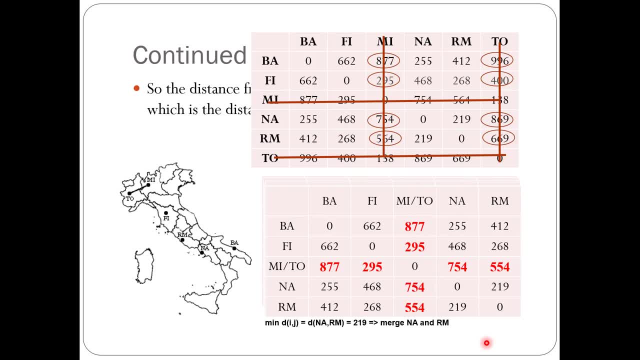 So we're going to go back to this matrix for a second, because we have to repeat the same process over and over again, And so in this row we have to find the new minimum distance in my matrix. Basically, we're trying to find what are the next two observations that are: 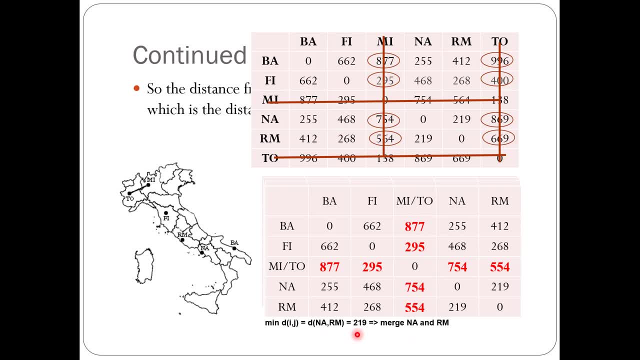 the closest together to be combined and form a cluster. If I look at this table, you see that Na and Rm, with the distance of 219, is the minimum value in this matrix. It's important to not confuse that with a single linkage method We're always at any stage, no matter. 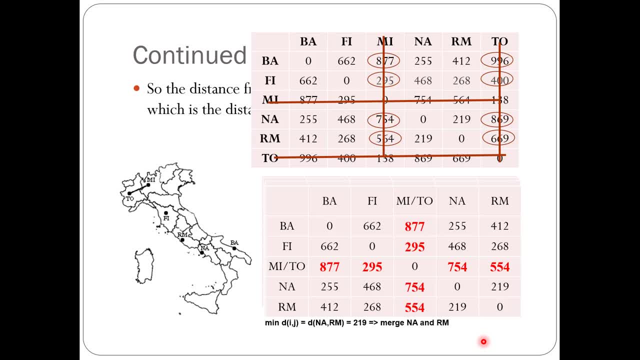 what method you're looking at. we're always Natürlich want to find the closest observation. However, when you update your matrix, then the method of calculating the cluster distances is the one that determines how you go about updating your distance matrix. I'm going to explain that more in the next round of this iteration. 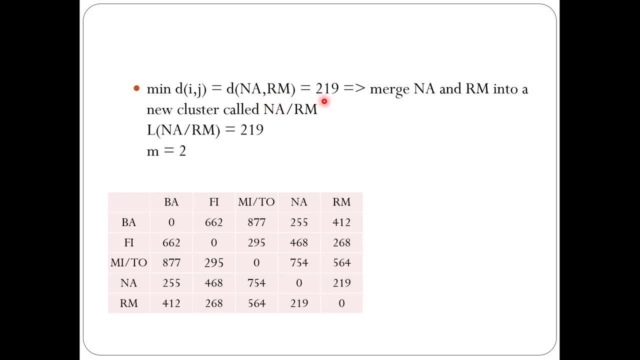 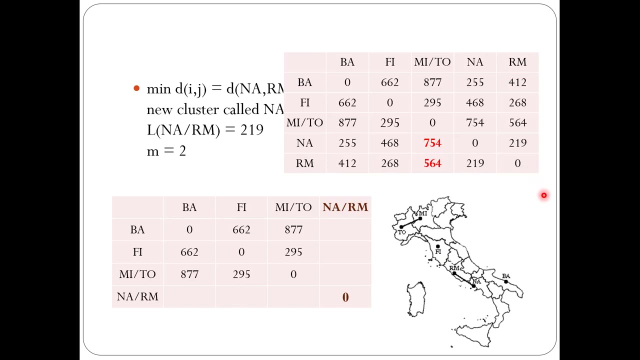 Alright. so we decided that Ni and Rm, with a distance of 219 in the second iteration, need to be merged to form a new cluster. I have to repeat the same thing. I combine NaRm and remove the NaRm column from the previous matrix, Both rows and columns. 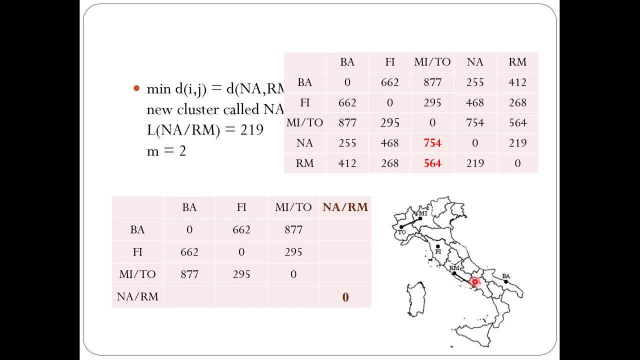 now in this graph here you see that NaRm are combined here. So now we have a new cluster and we have to update all these distances from this new clusters because previously all these distances are calculated to each of these observations separately. Now that I've found the closest two observations or NaRm to find the distance. 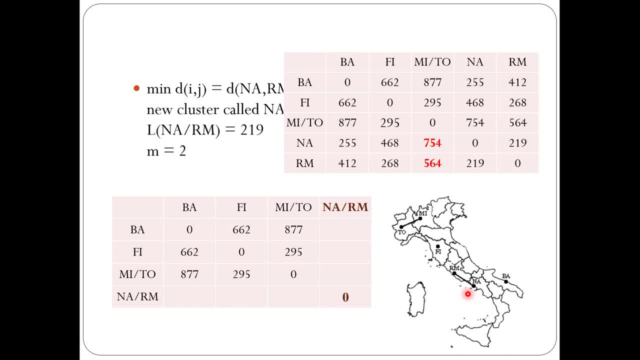 of all the other observations from this new cluster, I have to choose single linkage method. For example, let's go ahead and update the distance of this cluster from MITO. We have two ways to do this. We either have to look at the four distances possible and, among the four distances, choose the minimum distance. 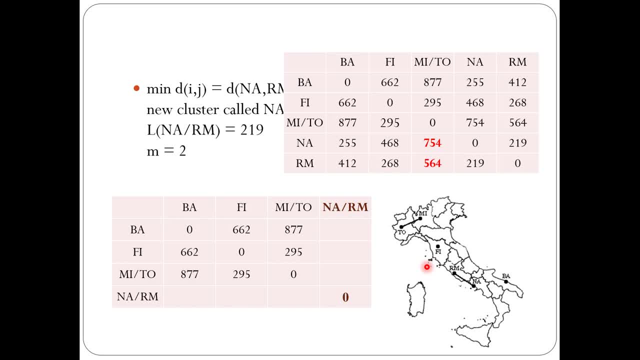 if you're going off of single linkage. If I had the complete linkage, then I had to choose the maximum distance. However, since we already know the distance of RM from MITO and NA from MITO, we don't really need to calculate four distances. We always can refer. 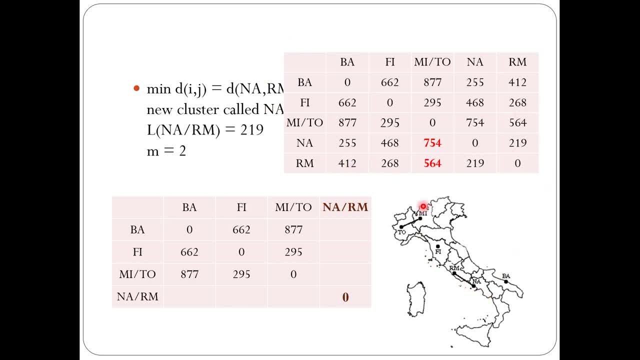 to the previous matrix and just look at two distances- the distance of MITO from RM and MITO from NA- to choose the minimum one based off of the single linkage method for updating our new distance matrix. So I'm going to go ahead and do that. The distance of NA from 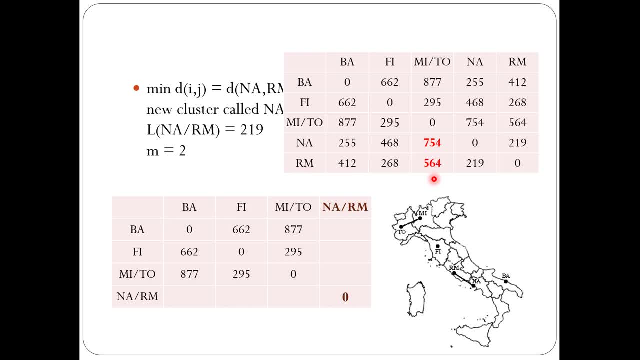 MITO is 754 and RM from MITO is 564.. The minimum of the two is 564.. So I'm going to put it here and here, because this is a symmetric matrix. Okay, so 564.. Now let's go ahead and 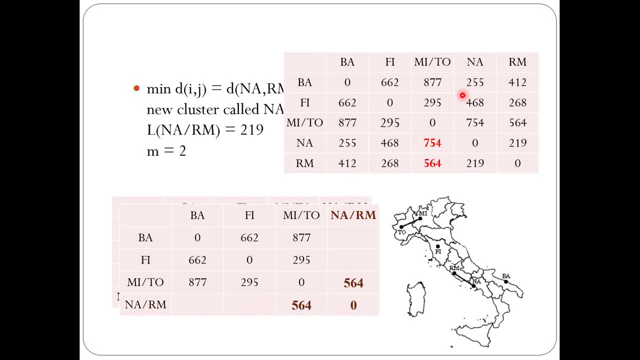 update the distance of NARM to FI. So if I look at the NARM and column FI, here is where I have the distances, So 468 and 268, the minimum between the two is 268, and I can update it in my new matrix. Same thing for the distance of NARM from BA to FI. I'm going. 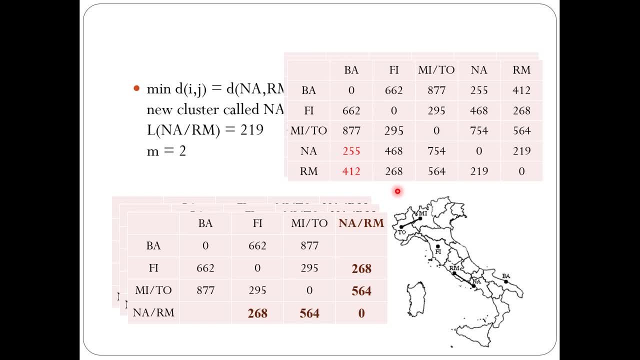 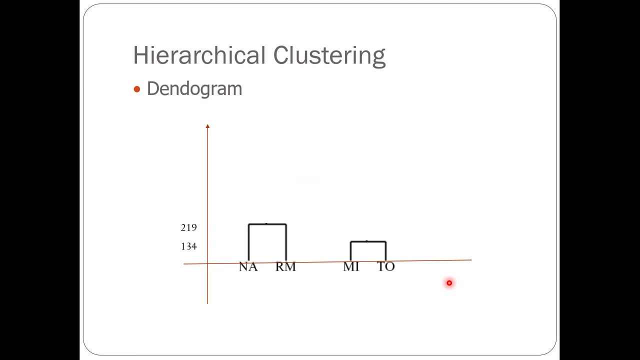 to put a new matrix and add a new matrix to FI. So this is our new matrix. Again, in this stage I combine NARM with the distance of 219.. I can show this in my dendrogram. Let's take a look at the dendrogram and see how we can build this new cluster in our dendrogram. 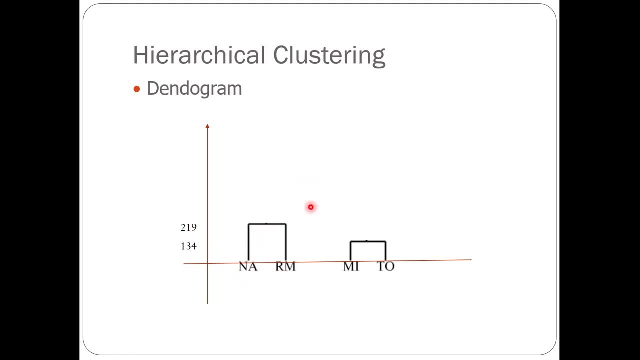 So NARM at 219 is the new addition to my dendrogram. Previously we had MITO with a distance of 134.. So let's move on to the next iteration, which is exactly the same as the previous two iterations In iteration 3,. 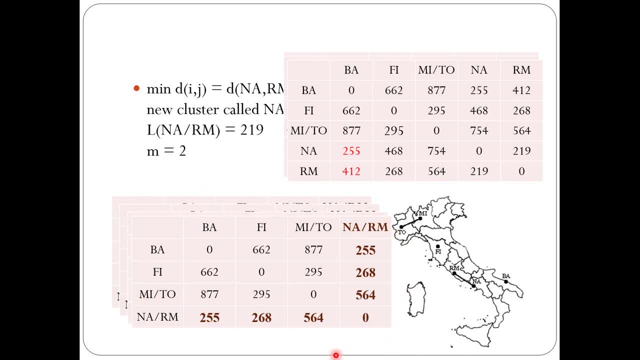 we find that the minimum value in this matrix here is 255, which is the distance of BA from NARM. So in the next table we have to remove BA and NARM both in rows and also columns and combine BA and NARM as our new cluster. So 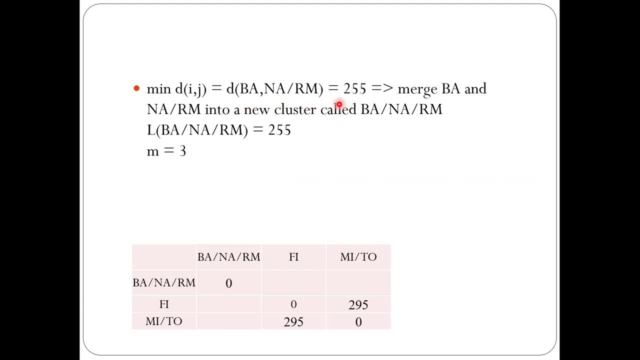 here is the summary: BA is going to be combined with the NARM with the distance of 255, and we are in iteration 3.. This is the new table which is created based off of the previous table, after eliminating NARM cluster and BA from the matrix and creating a joint column and rows for them. 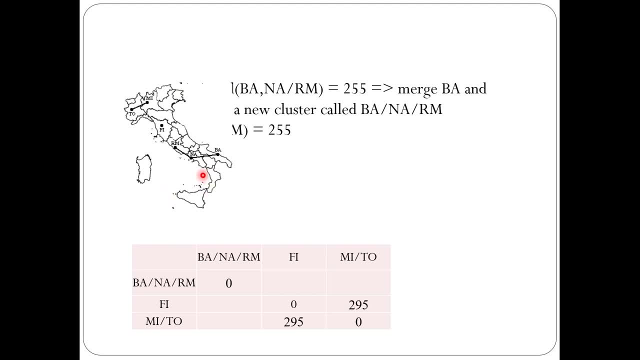 So here's the graph that shows how BA is combined with NARM. Let's take a look at the previous step matrix. So if I want to update this matrix again, I have to look at the distance of BA and NARM from Fi. 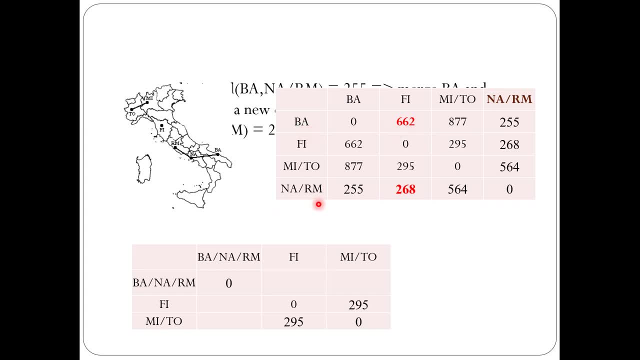 Basically I have to look at the distance of BA from Fi and NARM from Fi in the previous matrix and choose the minimum of the two, because we're looking off of the single linkage. So 268 would be the answer in my matrix. Now in the next step, 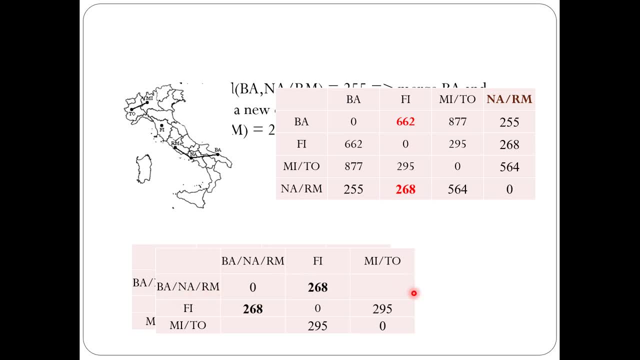 I want to update the distance of BA and NARM from MITO. So this time I have to look at the distance of BA from MITO and NARM from MITO, And between the two I choose the minimum one, which is: 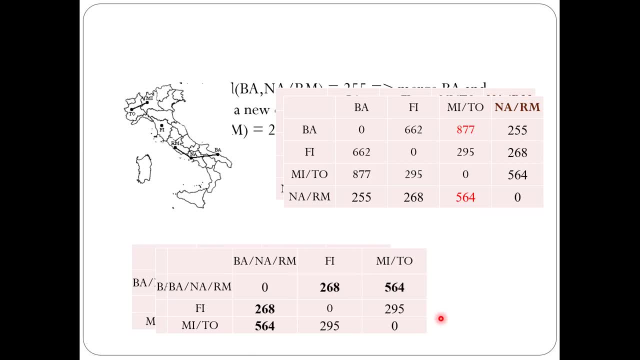 564.. Now that I have created the new matrix, I have to go to the fourth iteration and, as I said earlier, we continue this process until we get to a 2x2 matrix. Now, before we go to the next iteration, 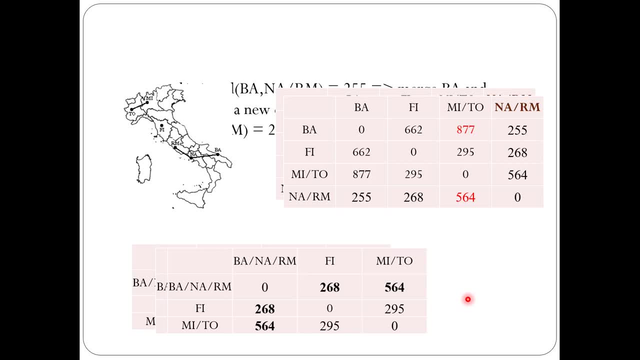 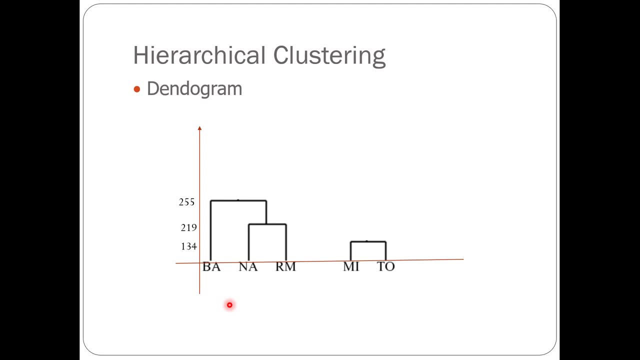 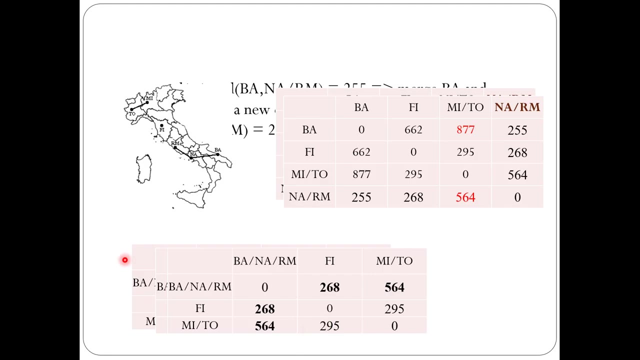 let's update our dendrogram by adding BA combination with NARM. BA is combined with NARM with a distance of 255.. So here's the new dendrogram: BA is combined now with NARM with a distance of 255.. Now in my new updated matrix the minimum distance is now between Fi and BA and NARM cluster. 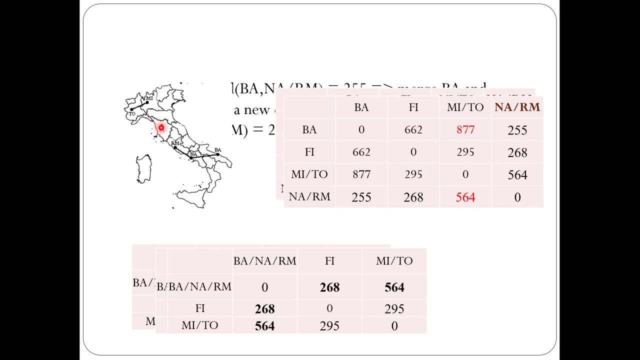 You can see it here. So basically, what we're going to do is combine Fi to RM and ABA cluster. This is the summary. BA and NARM is going to be combined with NARM. So basically, what we're going to do is combine Fi to RM and ABA cluster. This is the summary. BA and NARM is going to be combined with NARM. 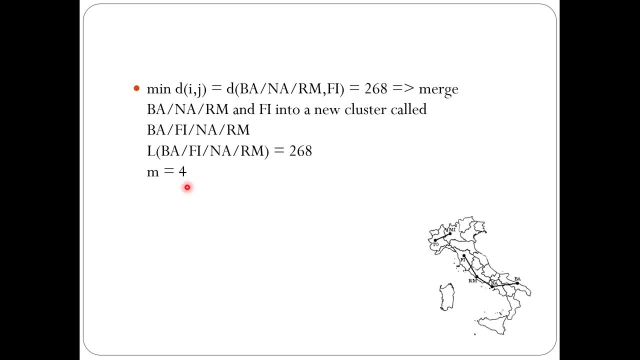 and we said only one, Hujin. So now, if I look at the distance matrix, I only need to find the distance distance of the new cluster, this new cluster from the MITO. so now, if I look at the distance matrix, I only need to find the distance of this new cluster, this whole new cluster from the MITO that we had previously. 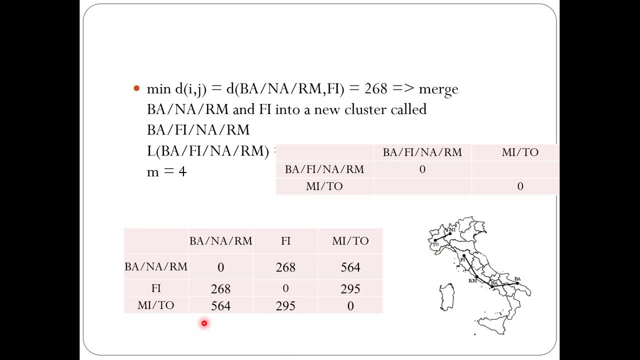 that we had previously. so now let's go ahead and see what's the distance here. so the distance of banarm from mito is 564 and the distance of fi from mito is 295. the minimum of the two is 295. now i can update my new distance matrix- 295, and i can go ahead and update my dendogram. so if i 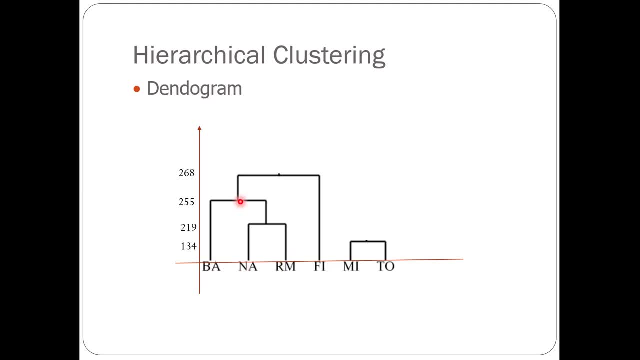 look at my dendogram. here i can combine this b, a, n, a, r, m cluster with fi with a distance of 268. when we get to this point where we only have two clusters, then we go ahead and combine the two clusters as well and finish our dendogram. if you look at the distance matrix, the distance of the 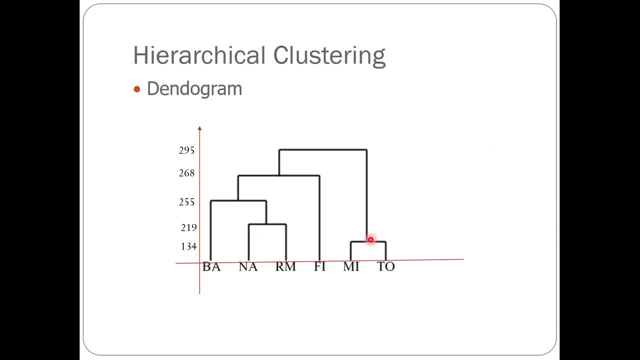 final two clusters is 295. so now i have combined these two clusters with a distance of 295.. a few things here. first, the dendogram has a maximum dendogram value of 16.65, which is the minimum of dendogram. First of all, we know that the length of this bar here shows how far apart two clusters are from each other. 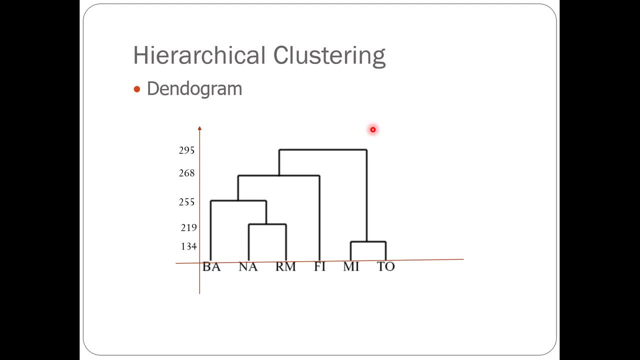 The higher this length, obviously the more apart two clusters are from each other. Now how do I use this dendrogram to perform the grouping of observations? To define the number of groups, I have to create horizontal lines that hit the vertical lines. 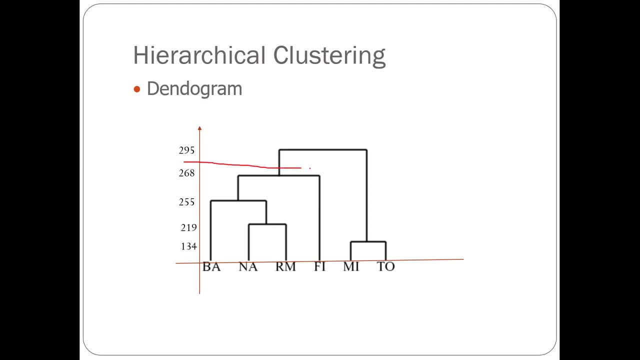 For example, if I want two groups, I have to draw a vertical line that hits the lines in two parts, And now I have created one cluster right here and one cluster right here. So if I want to divide these observations in two groups, one group is going to include B-A-N-A-R-M-F-I. 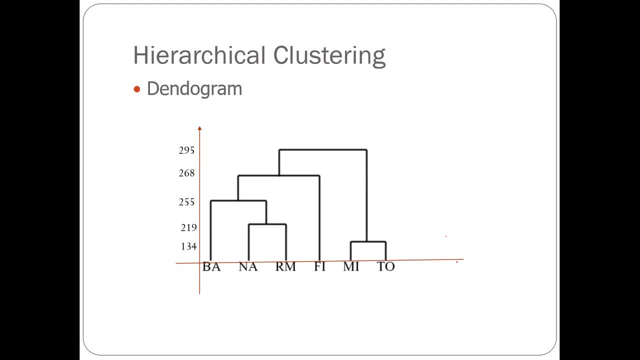 and the other one is going to include M-I-T-O. Now let's say we want to create three clusters and divide these observations in three groups. Then I have to draw a horizontal line that hits these Vertical lines at three parts, And each of these vertical lines lead me to a new cluster. 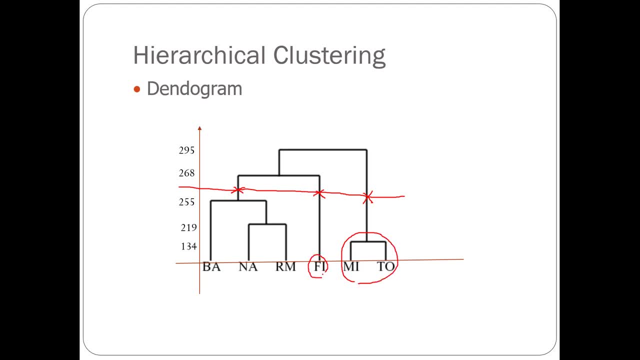 So M-I-T-O is one group. Coming off of this line, you get F-A, And coming off of this line, you have B-A-N-A-R-M. So I have three groups and each of these groups are clearly defined using my dendrogram. 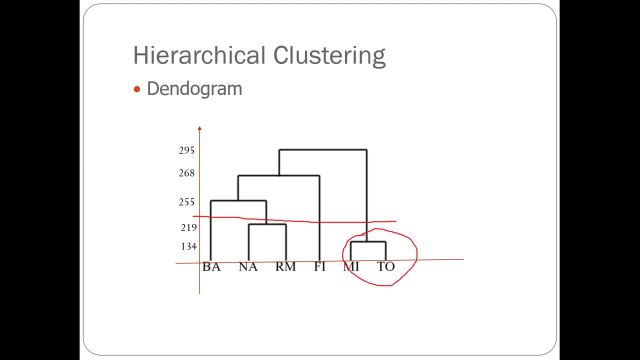 Now, if I want to create four groups, then you have one group here, one group here, one here and one here, So now you have four groups of observations. So the good thing about hierarchical clustering is that you don't have to have a predefined number of groups to start your clustering method. 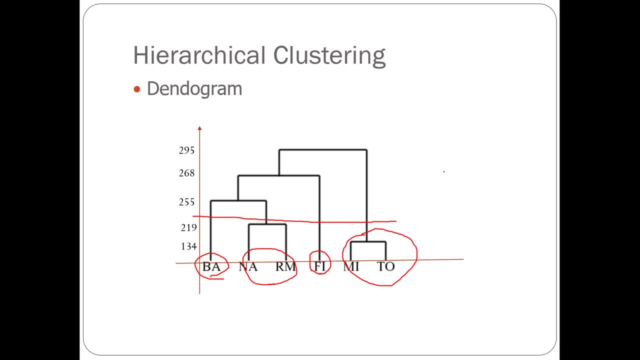 But that wasn't the case when we did the k-min clustering. In k-min clustering we had to know how many groups we're going to have in the end, and that determined the k at the beginning of our method. So this is one of the advantages of hierarchical clustering. 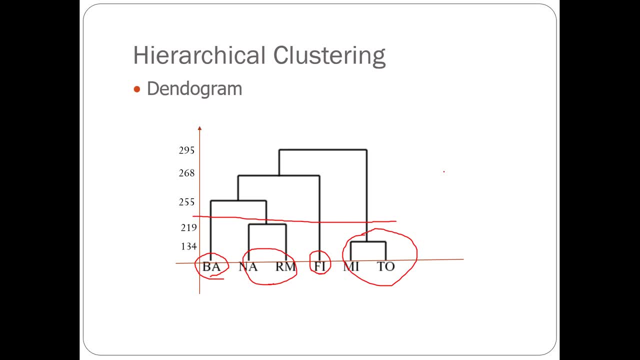 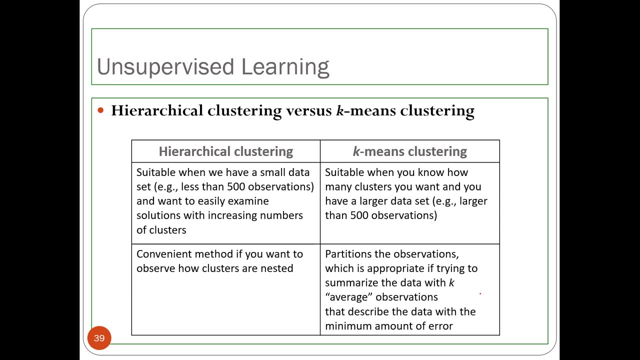 that you can go ahead and create your dendrogram and, in the end, define how many groups you want to divide your observations into. Let's go ahead and do a comparison between hierarchical clustering and k-min clustering. Hierarchical clustering it's going to be a little bit more computationally extensive. 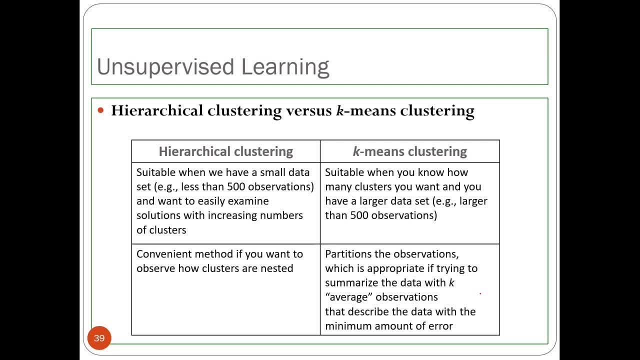 because you have to create a matrix of distance at the beginning. So if you have millions of observations, you have to create a million-by-million distance matrix at the beginning of your calculation, which is computationally intensive. However, it has the advantage of not defining the number of clusters at the beginning. 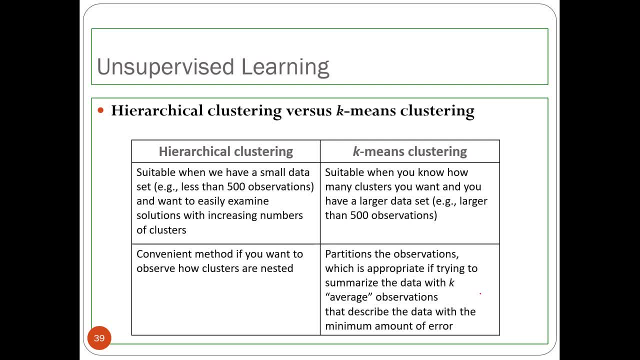 which is not the case when we have the k-min clustering. Another advantage is that it's very easy to see how your clusters are nested and how apart they are in terms of their distances, by looking at them as a very nice visual graph. However, k-min clustering also has some advantages. 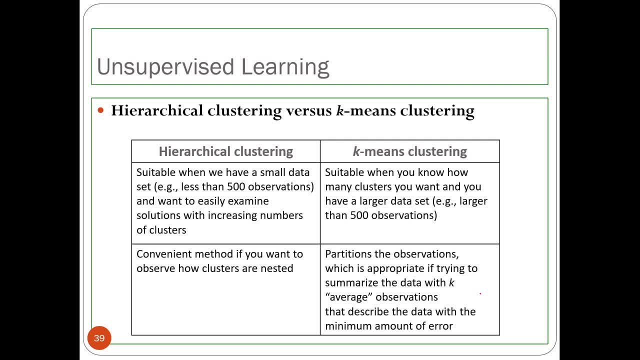 k-min clustering is obviously better when you have more observations. Let's say, if you have 500 observations. in hierarchical clustering, you have to make a 500-by-500 initial distance matrix to start with. However, in k-min clustering, because you define your k at the beginning, 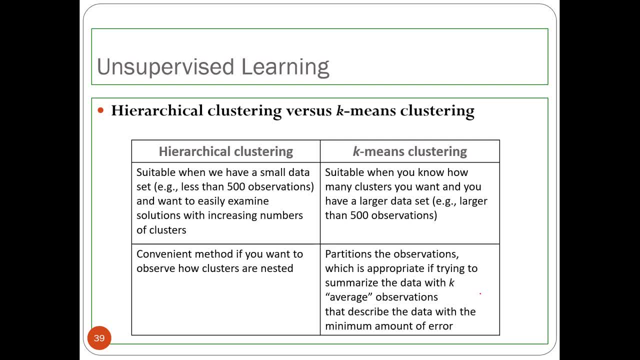 let's say your k is 3, you only make a 500-by-3 distance matrix at the beginning, which is much smaller than 500-by-500.. So it's typically better if you're dealing with a larger number of data. 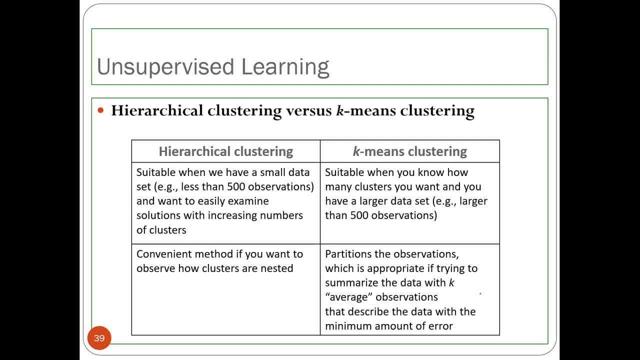 And also k-min clustering has advantage over hierarchical clustering in terms of summarizing the data better and averaging your observations in each group, and typically lower amount of error in comparison with hierarchical clustering. With this, our lesson in hierarchical clustering has concluded. Thank you for watching.